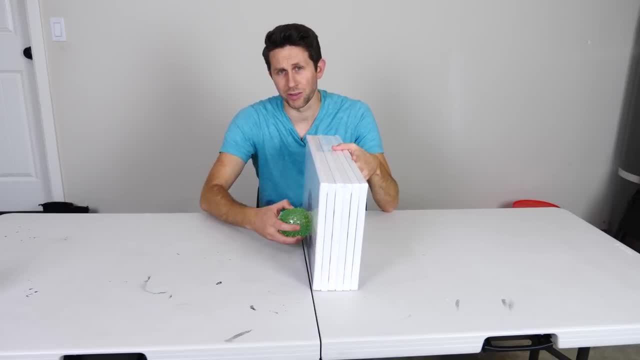 The only way it could do that is if it went around it or it broke through it. But if you say that the particle is going to move in a straight line and it's not going to break through it, it means that in classical mechanics, classical physics, 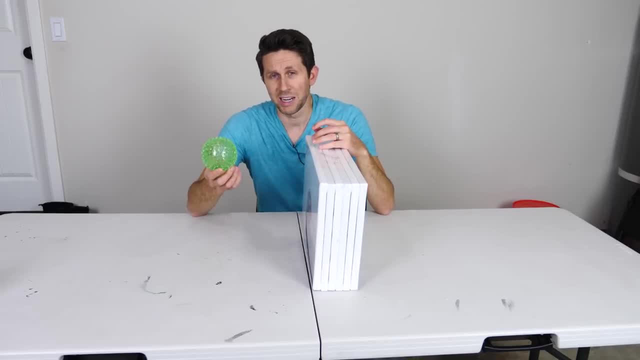 there's no way it can get through it. But what's weird is if you shrink everything down to a smaller scale, that's not the case. So, for example, let's again say this is now the size of an electron. Well, even on the quantum scale, if something's pretty thick, 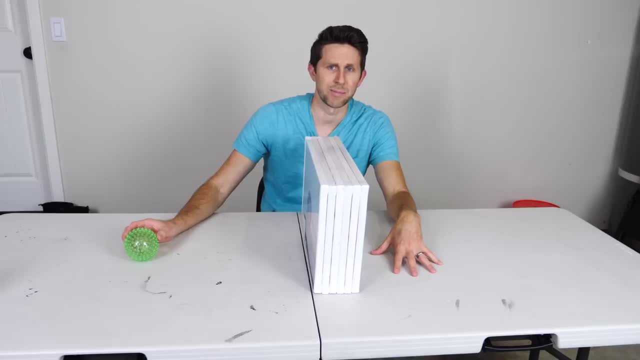 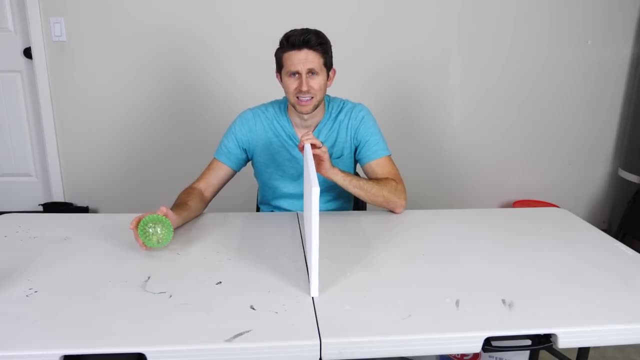 you're going to get a pretty close to zero probability that you're ever going to measure the electron on the other side of this barrier. But what happens is if that barrier becomes very thin, there becomes a non-zero probability that you'll find the electron on the other side of the barrier. 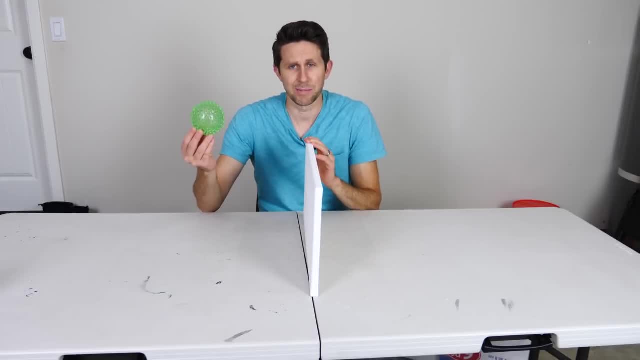 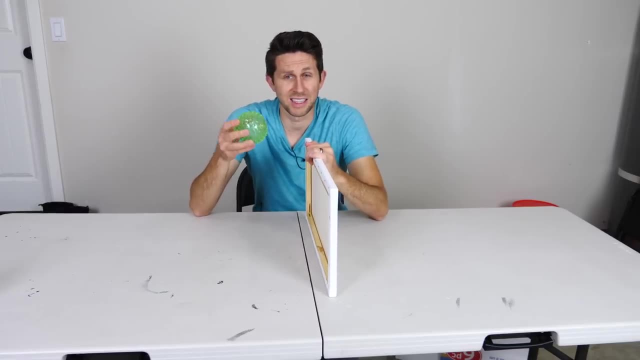 without ever having broken the barrier. So what that means is on a quantum scale, sometimes electrons can just go through stuff. And quantum tunneling is interesting because no matter how impenetrable your barrier is, it doesn't matter because there's always some non-zero probability. 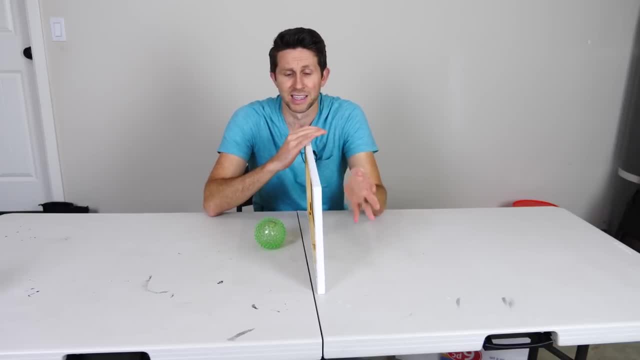 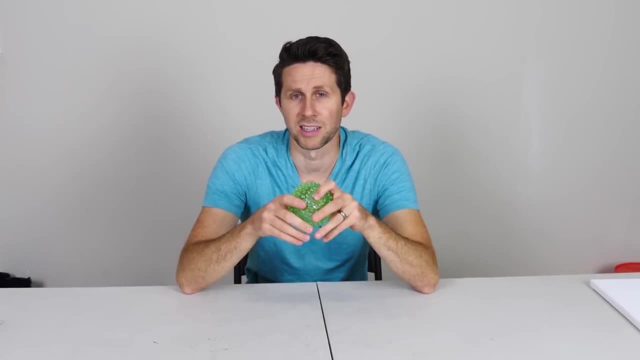 that a particle's going to end up on the other side of it when you measure it, as long as this barrier is thin enough. So the particles that we're going to be using for our experiment are photons, And the impenetrable barrier that we're going to be using is a reflective surface. 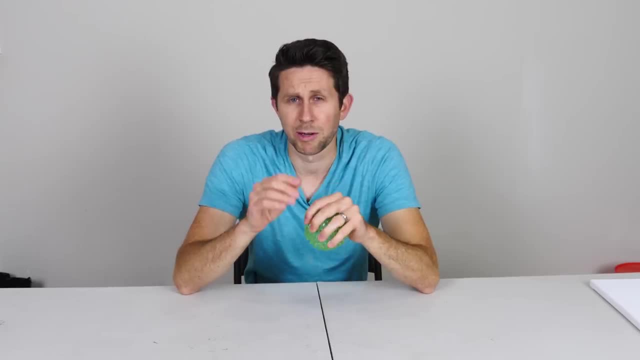 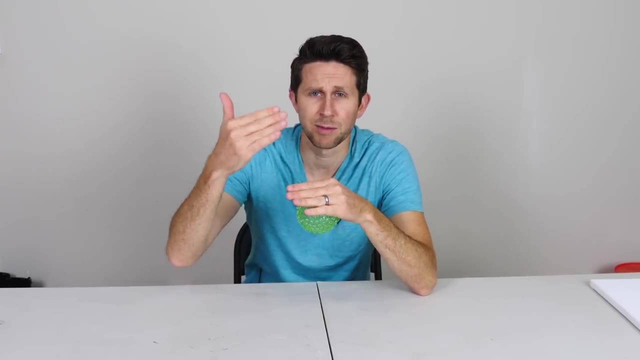 Now, instead of using a mirror for our reflective surface, I'm going to be using the boundary between water and air. Now, the boundary between water and air can act as a 100% reflective mirror because of the differences in the index of refraction of water and air. 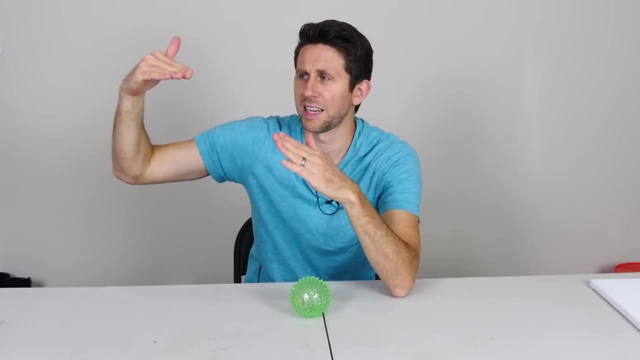 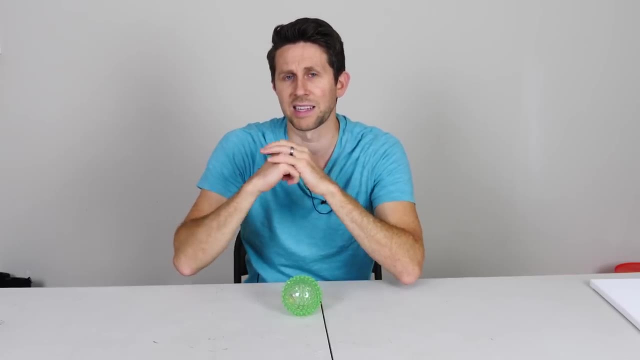 So when you're past a specific critical angle and you're shining light out of water, what happens is that light doesn't actually leave the water, but it just reflects off the surface and goes back into the water, And this is called total internal reflection. 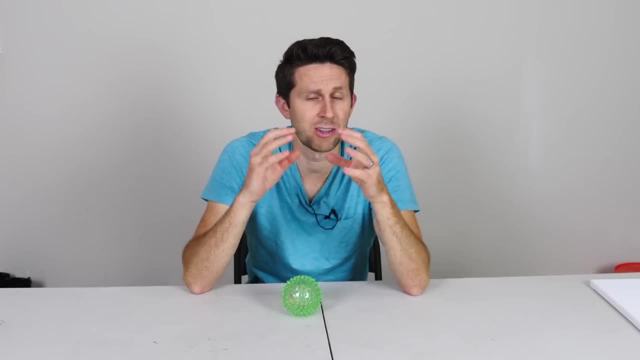 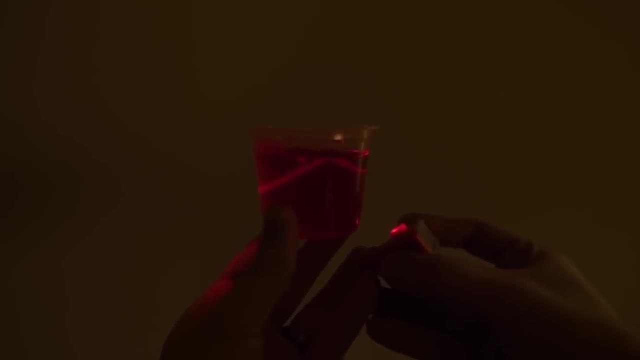 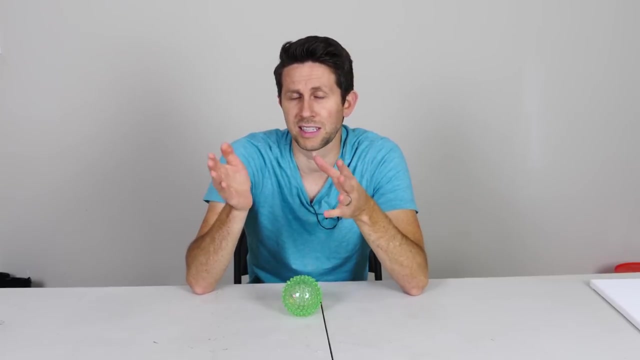 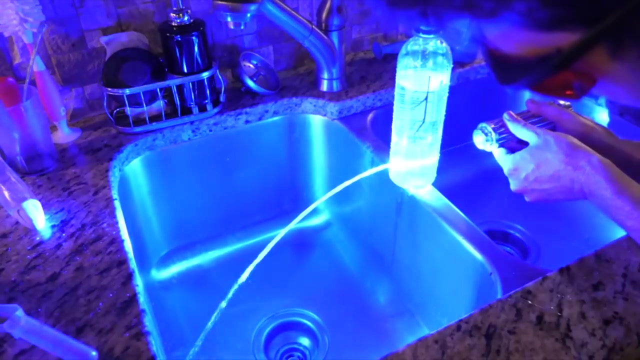 This is how fiber optic cables work as well. You can show total internal reflection even just using some jello and a laser. You can also show this total internal reflection using a laser with water pouring out of a spout. Look how the laser just stays with the water. 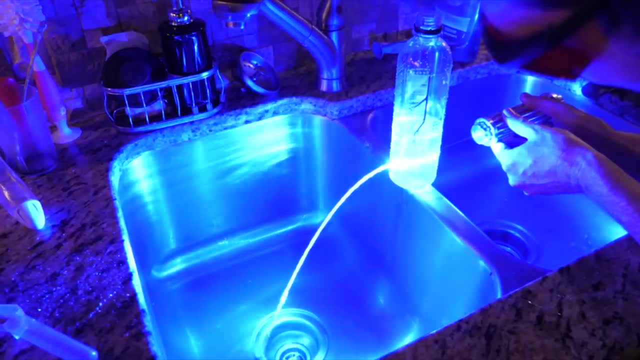 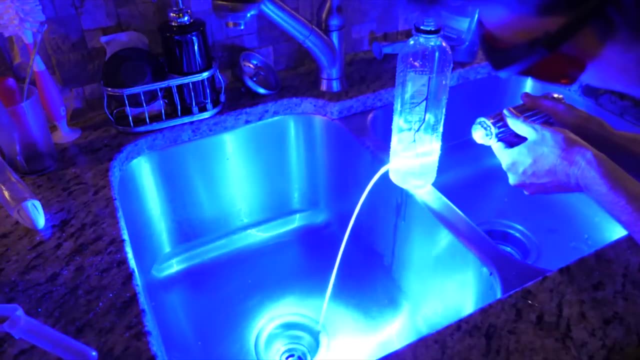 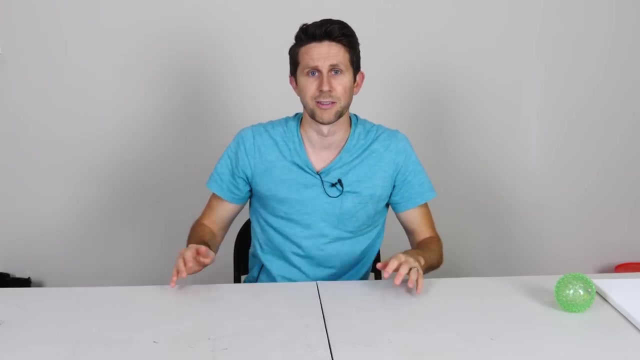 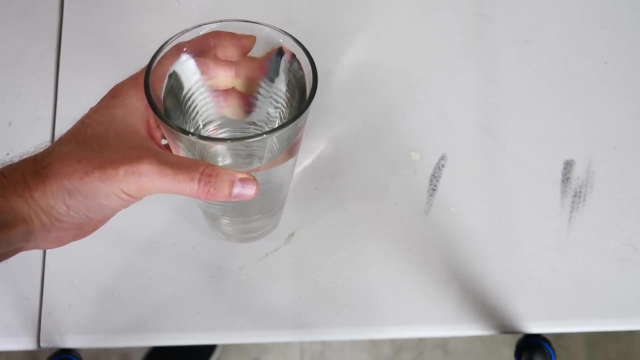 Look how the laser just stays with the water. Now another way to see this total internal reflection is just to look into a glass of water. Let me show you Now. here's a really easy example of total internal reflection. Notice that as I hold the glass sideways, you can see my fingers easily on the other side of the glass. 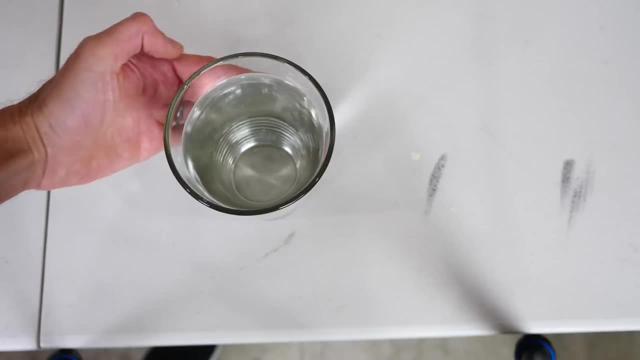 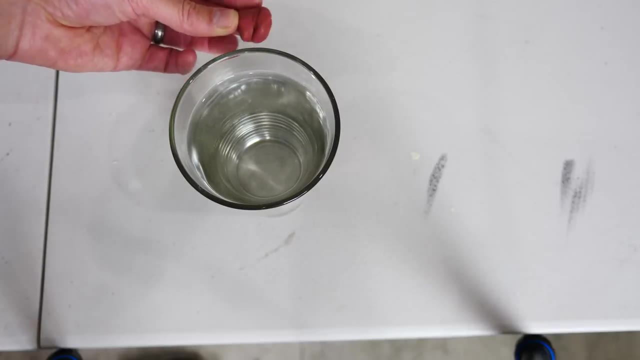 But when I turn the glass upright, suddenly the sides of the glass become like a mirror. You can't see anything outside of it. So as I move anything down the side of the glass, you can see it, But as soon as it dips below the surface of the water, suddenly you can't see it. 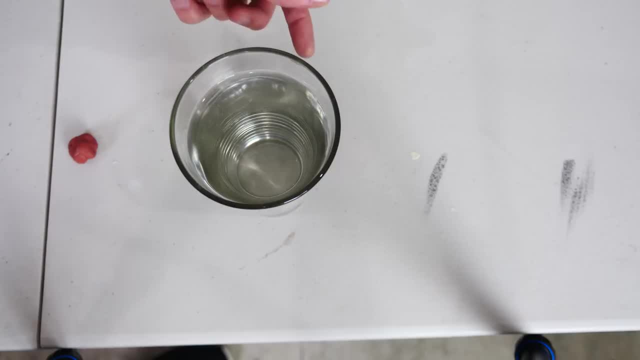 So basically, this water glass boundary here is acting like a barrier. It's not letting any light pass through this, So no light is getting from my finger to the outside of the glass up through the camera. You can see it completely blocks my hand here. 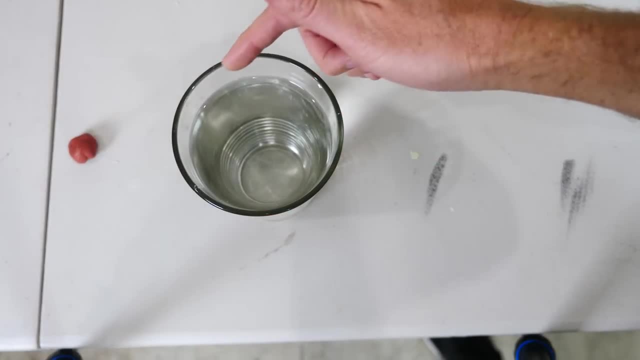 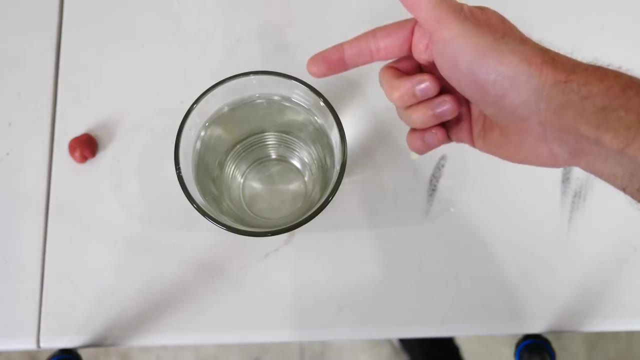 And again, the reason this is happening is because the water and the glass have a fairly different index of refraction than the air around it. And what happens in this case? because the air has a lower refractive index than the glass and the water. it means that the probability of finding a photon outside of here 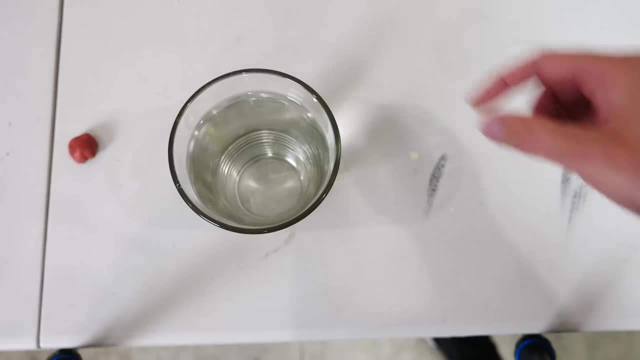 exponentially, decays to zero quite quickly. So in this case the boundary is actually the air around the outside of the cup. So the photons coming off of my finger don't make it through the camera, because there's a boundary of air in between my finger and the camera. 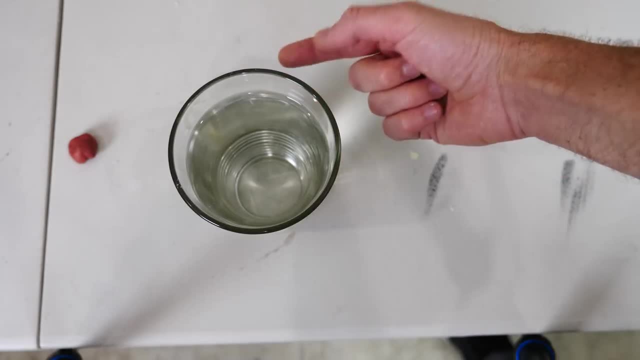 And so you can't see the photons coming from my finger. But it turns out, if you can make that boundary small enough, if you can get that layer of air small enough, you actually can see the light. So the photons from my finger can actually. 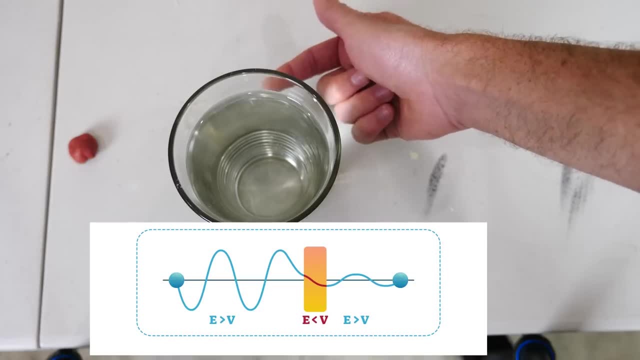 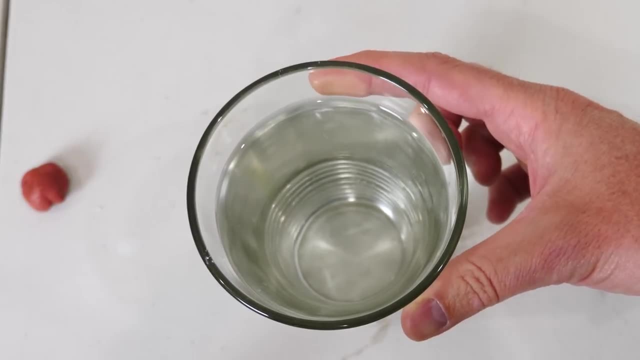 quantumly tunnel through that boundary layer of air and get to the camera. So when I touch the glass, you still can't see my fingers. That's because, even though there's only a tiny little bit of air, even when I'm pressed against it, you can't see my finger. 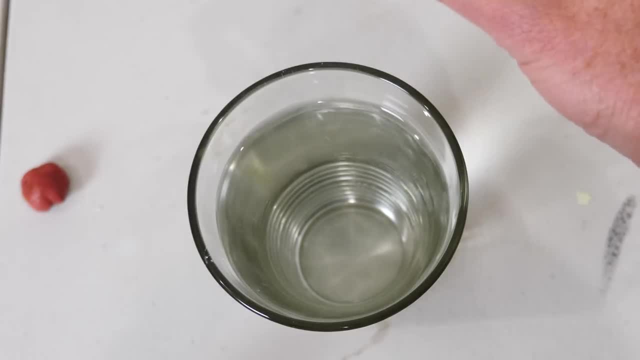 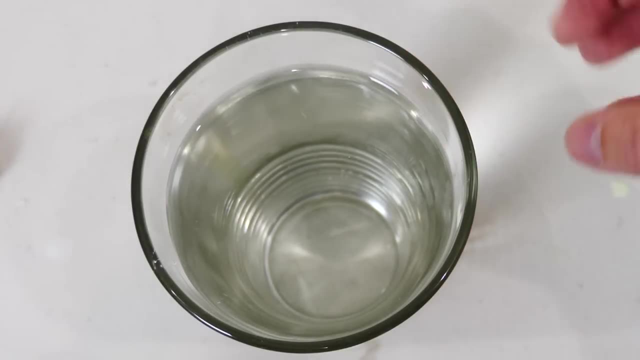 Because even though there's just a tiny little bit of air, it's still a thick enough boundary that it acts like a barrier to the photons coming off from my finger. But now watch what happens if I press really hard and try to reduce that air layer. 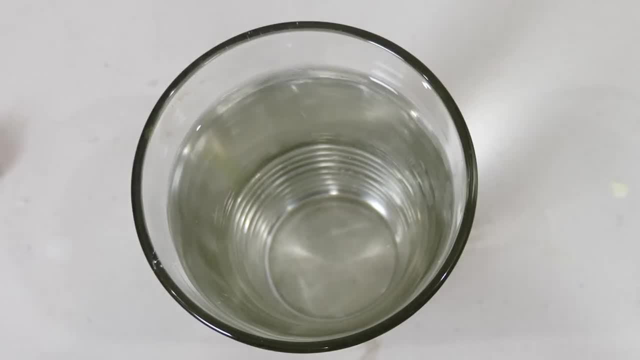 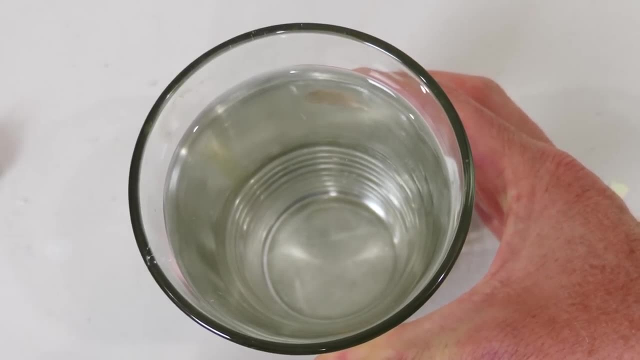 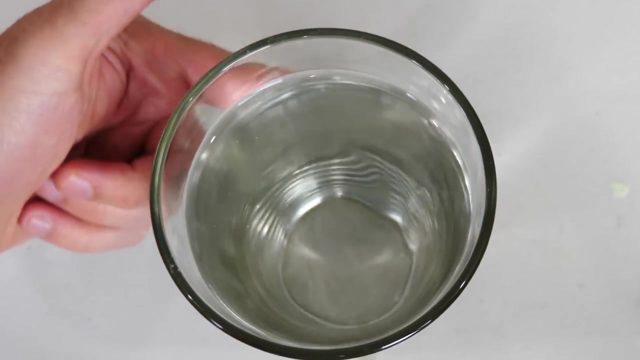 in between my finger and the glass to as small as possible. It turns out that you actually can start seeing my finger, Do you see it? So when I just hit the glass like normal, see, I can push the glass. you don't see my finger. 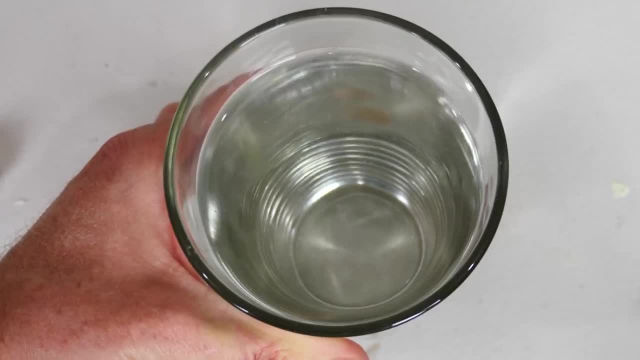 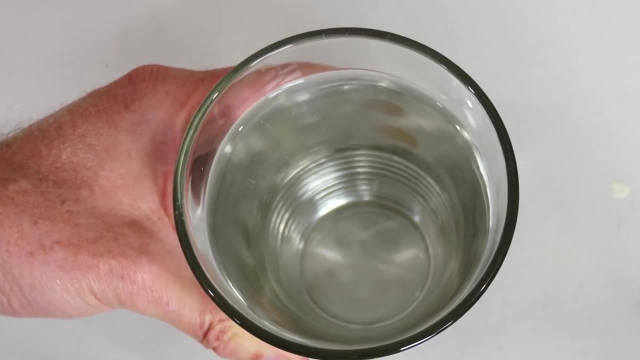 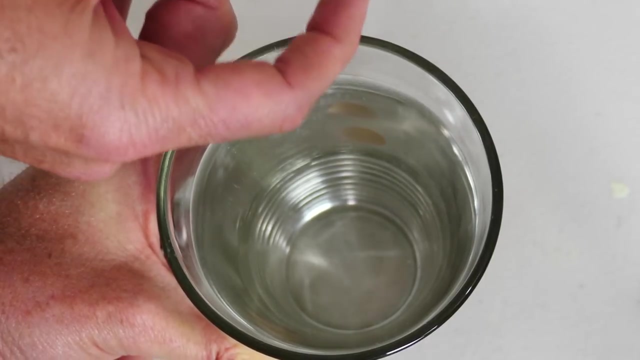 But if I press really hard now you can see my fingerprints and my finger on the glass. So this is actually a great analog of quantum tunneling. So the only way these photons are getting through this barrier is because I've reduced the barrier of air to a small enough thickness. 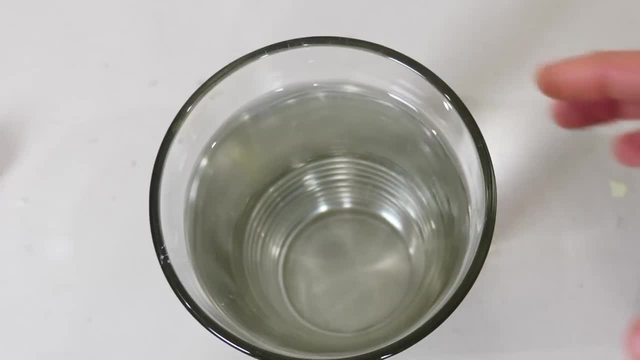 that the photons actually tunnel right through it. Another way to do this: instead of pressing really hard with your finger, you can reduce that boundary of air in between there just by getting your finger wet. So now my finger's wet. So instead of air in between there, 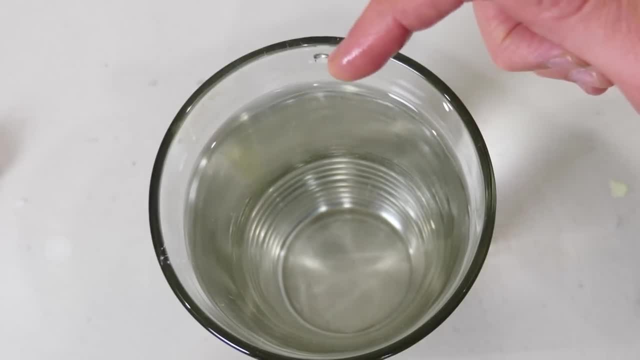 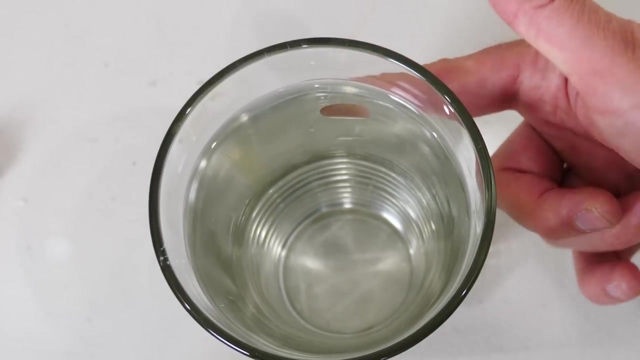 there's water and the water has around the same index of refraction as the glass and the water. So then you can easily see my finger. So having that water on my finger, I can easily see my finger. So having that water on my finger reduces that layer of air very quickly. 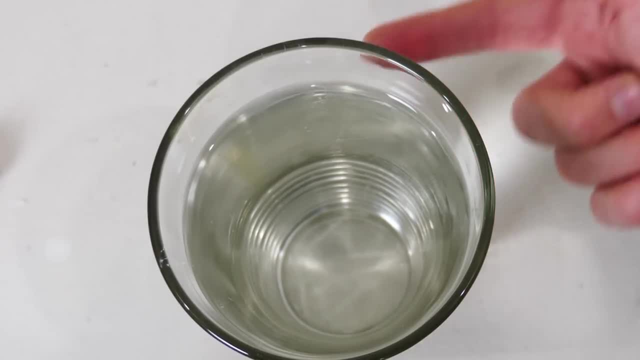 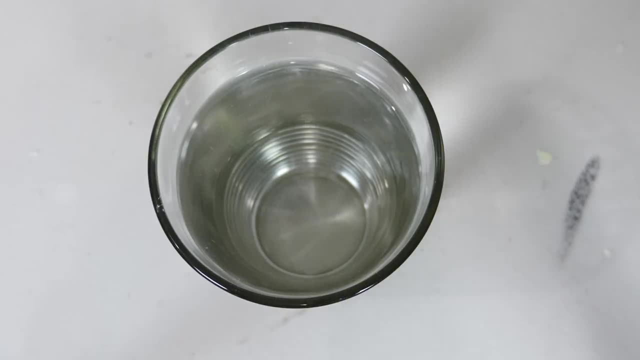 so that the photons from my finger can get from my finger to the camera. Now this happens with any object, not just your finger, and it doesn't even have to be wet. So I have just some silly putty here. You can see, if I push it hard enough, you can see it on the other side of the glass. 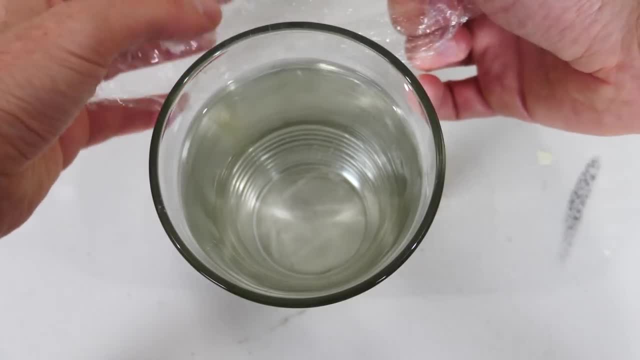 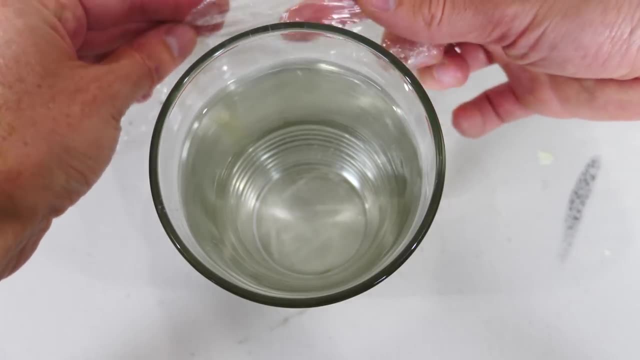 But if I don't push it hard, you don't see it. And also to show that it's not just my finger being wet that's getting it to show up on the other side of the glass, I'll put this barrier in between. 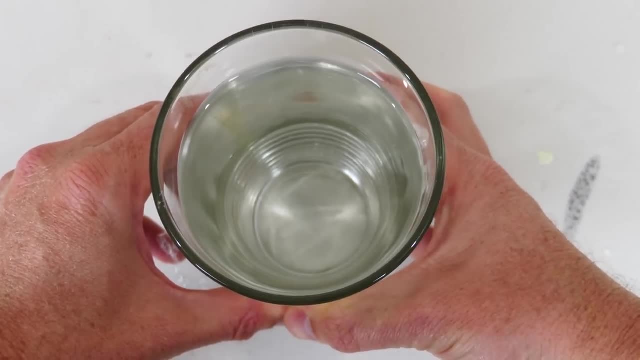 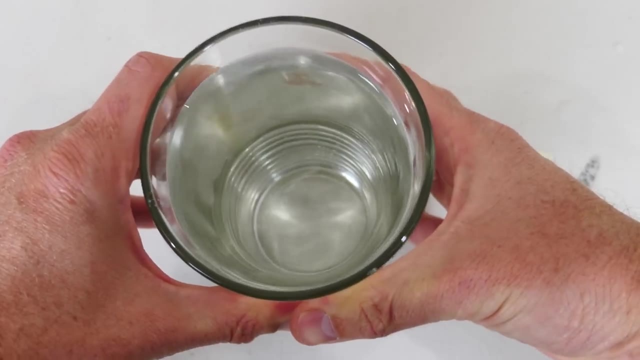 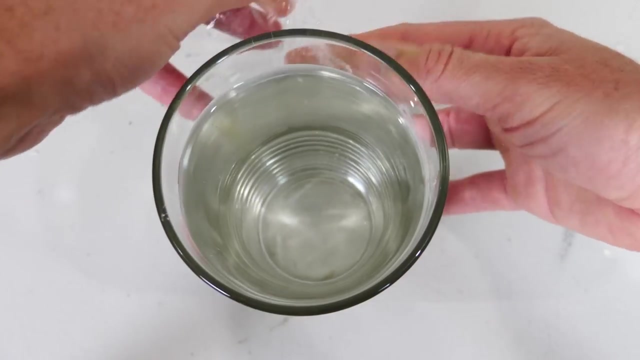 But if I push hard enough and squish the air out, you can still see my finger. So again, it's not because my finger is wet, my finger's not even touching the glass. it's because I'm squishing out enough air. 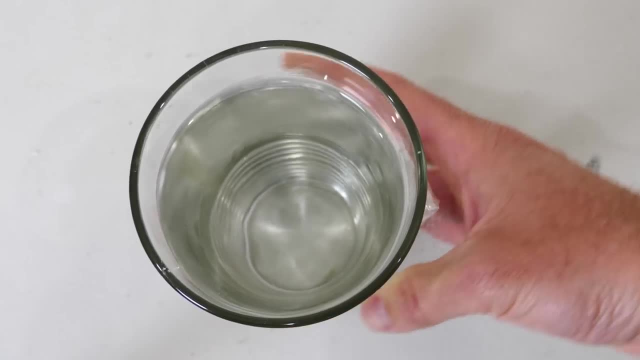 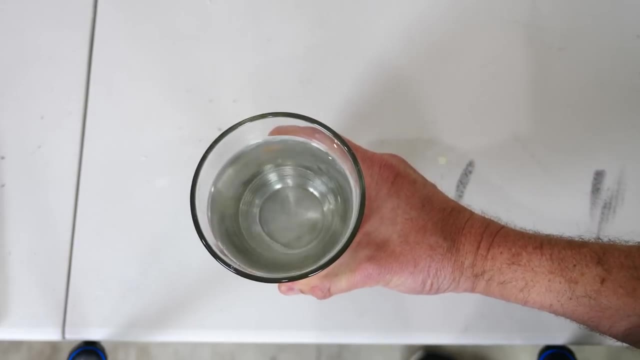 and so it no longer acts like a barrier, and so the light can pass through. So next time you're at a restaurant and you notice that you can only see your fingers on the glass when you're holding it tight, you can start up a nice conversation about quantum mechanics at the table. 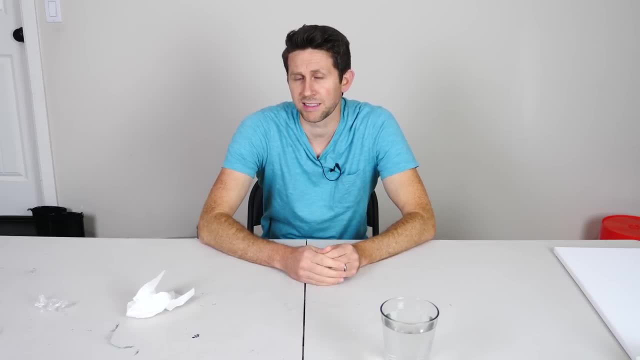 Now, the experiment that I've done here today was with photons, but you can actually do the same thing with electrons as well, So even real electrons can tunnel through stuff. Except it's just a lot harder to show in experiments because electrons have a lot smaller wavelengths than photons. 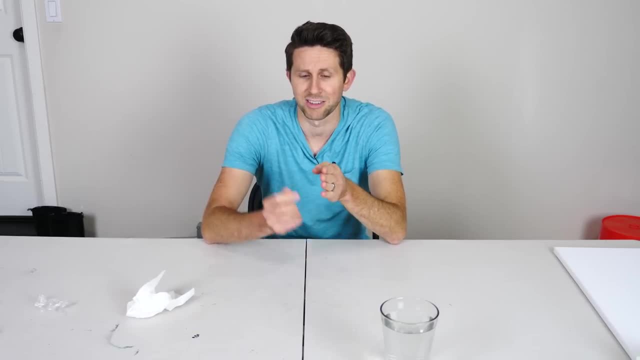 And so, basically, you need something that's extremely thin in order to show how electrons can tunnel through it. Now, this can actually pose a problem in the semiconductor industry On the scale that we're now building transistors, when you have two conductors that are close together. 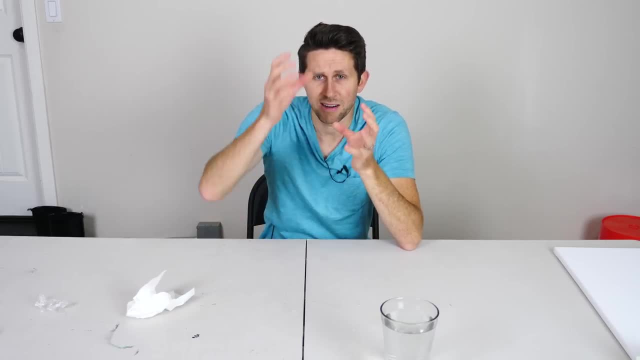 and some non-conductive material in between. no matter how good of a resistor that non-conductive material is, it means that some electrons can still get through it, no matter what you do. In fact, even if you had a problem, you could still get through it. 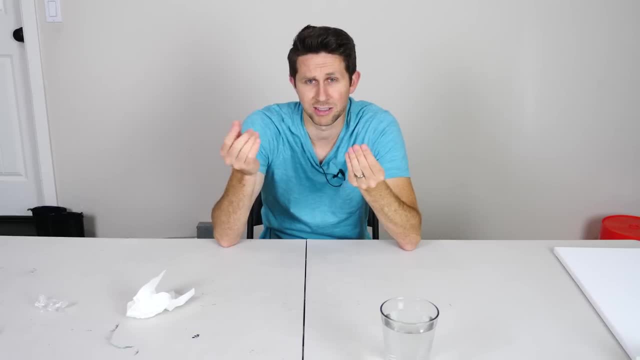 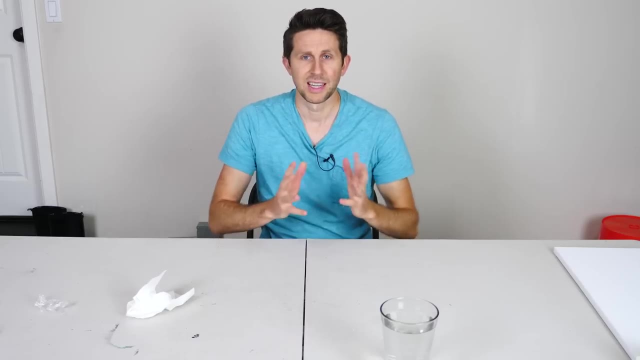 If you had a perfect resistor. if you get these two conductors close enough, some electrons will just go right through it, even though they never actually went through the non-conductive material. And thanks for watching another episode of The Action Lab. I hope you enjoyed the video. 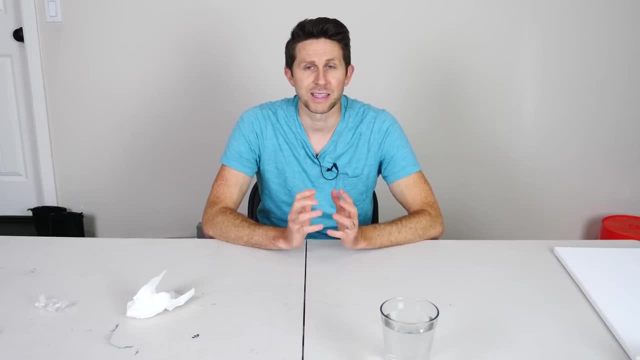 If you did remember to hit the subscribe button, and remember to hit the bell so that you can be notified when my latest video's out and get right on watching it And check out theactionlabcom for the Action Lab subscription box. You can check out the link in my description for the Action Lab experiment book. 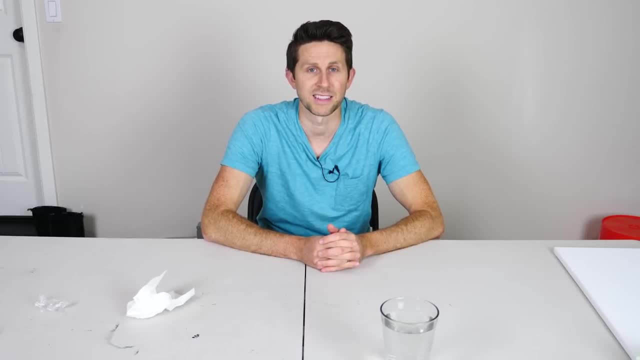 called Extreme Garage Science, And thanks for watching and I'll see you next time.